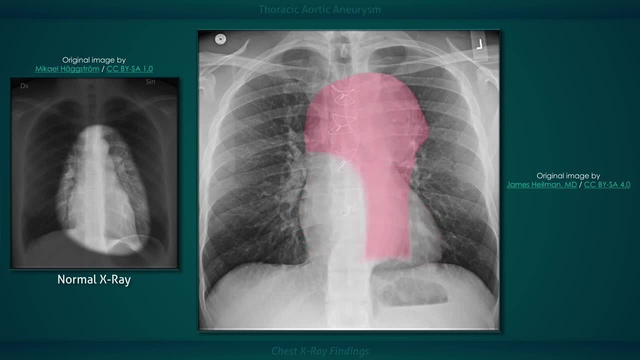 Now let's address the wider mediastinum. The large mass has a homogeneous density with sharp margins, and it extends out laterally on both sides. The ascending aorta, the aortic arch and the descending aorta are all dilated. 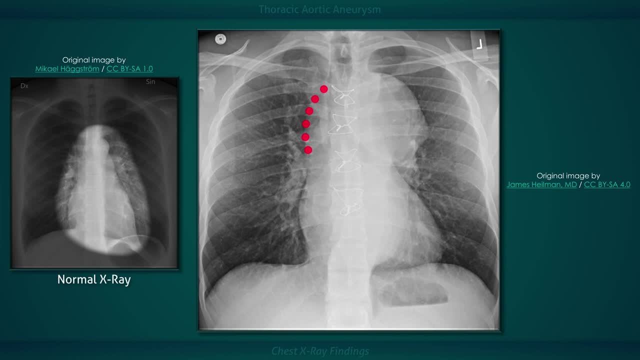 When the aneurysm only involves the ascending aorta, the bulge typically appears on the right side of the chest, and when the dilation is extensive, the ascending aorta may form the upper right border of the cardiac silhouette. Dilation of the descending aorta, as may be expected, results in a left-sided bulge. 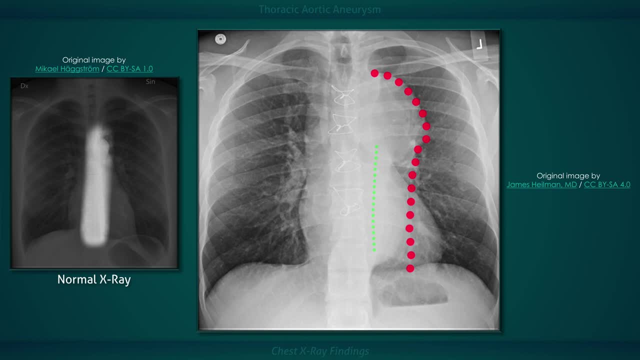 The absence of the descending aortic shadow in its typical location provides further evidence that the mediastinal widening is due to aortic disease. Calcification of the outer wall can occur, particularly with acquired aneurysms, but it is not present in this case. 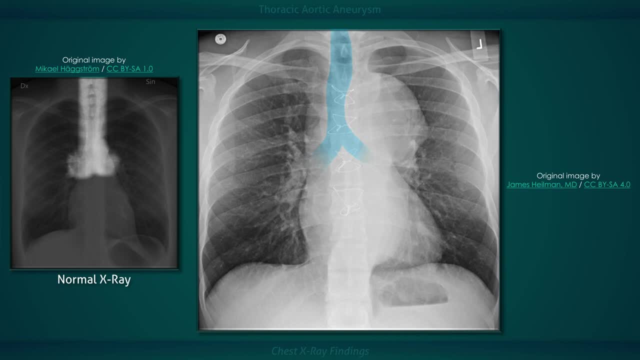 Finally, take note of the convex point of the trachea. The aortic arch is a structure in the superior mediastinum and when it is significantly enlarged it can displace the trachea rightwards and the left main bronchus downwards. 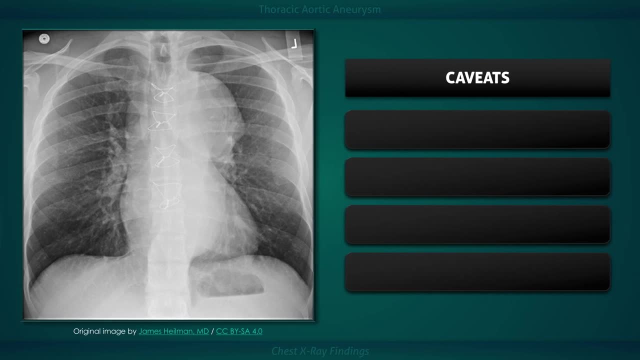 When considering the possibility of a thoracic aortic aneurysm, you should keep in mind a few caveats. A rotated x-ray can give the appearance of mediastinal widening. The aorta can be quite tortuous and elderly Mediastinal masses such as a thymic tumor can appear very similar. 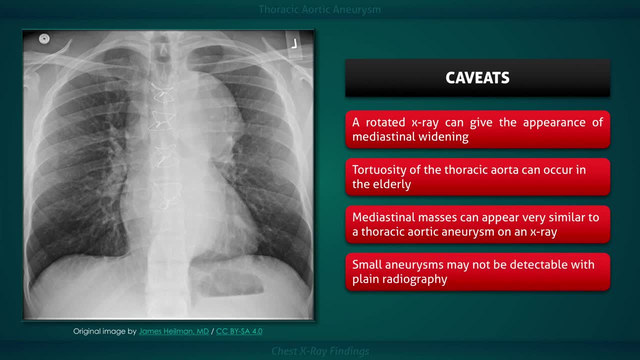 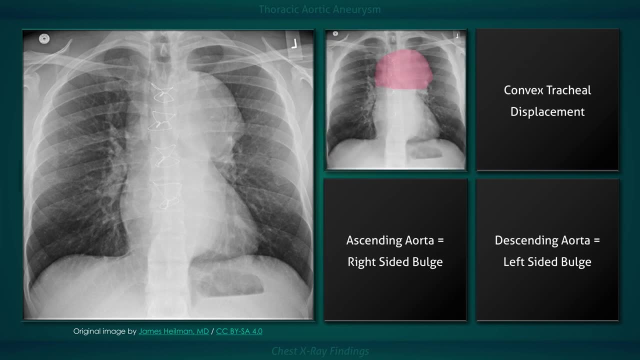 And small aneurysms may not be detectable with plane radiography. Now for a quick review. The most common chest x-ray finding in a patient with a thoracic aortic aneurysm is mediastinal widening. Calcification of the outer wall can occur, but it is relatively uncommon. 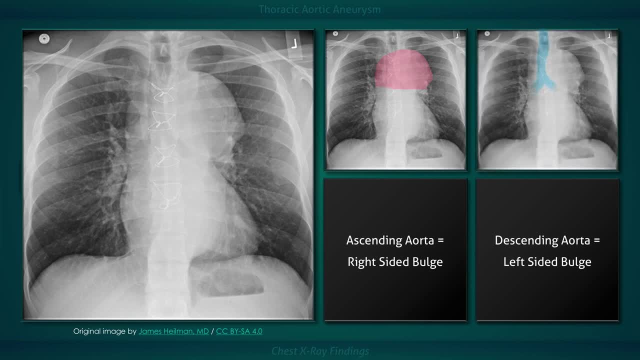 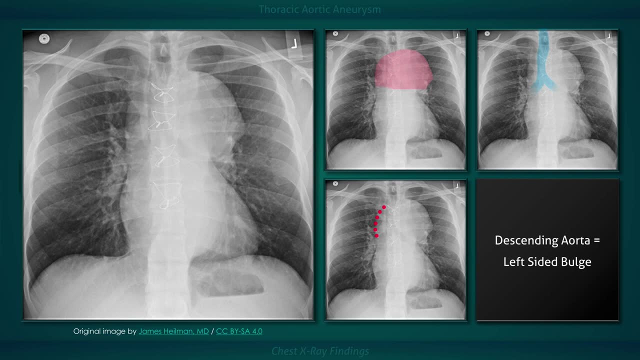 Large aneurysms can cause lateral displacement of the trachea and inferior displacement of the left main bronchus. Aneurysms that are limited to the ascending aorta typically cause a right-sided bulge and, when large, can form the upper right border of the heart. 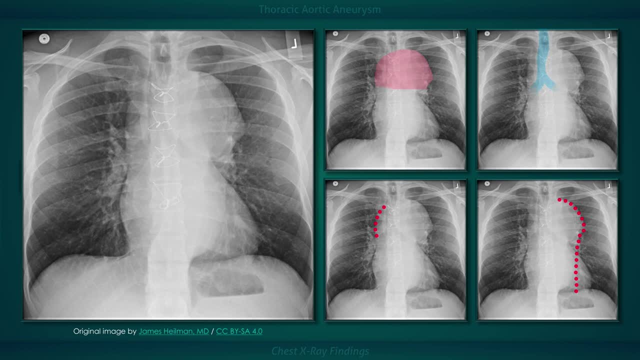 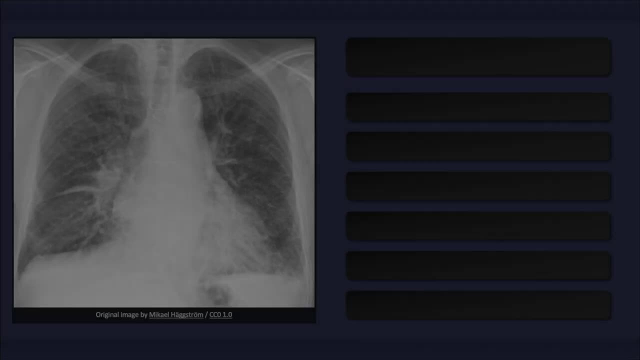 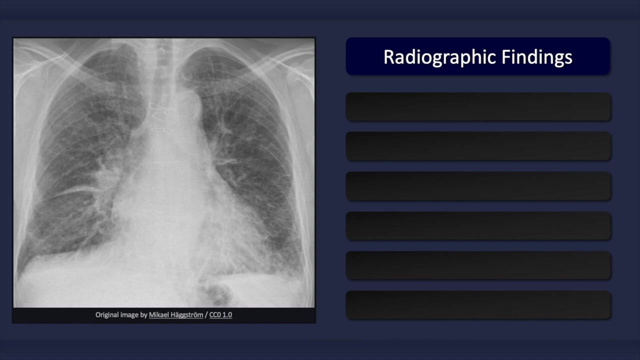 And aneurysms that are limited to the descending aorta typically cause a left-sided bulge. Congestive heart failure can produce a myriad of findings on plane chest radiography. Which findings are present depends on the severity of the patient's condition. 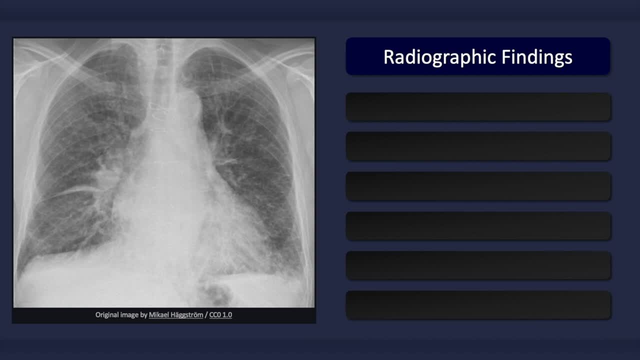 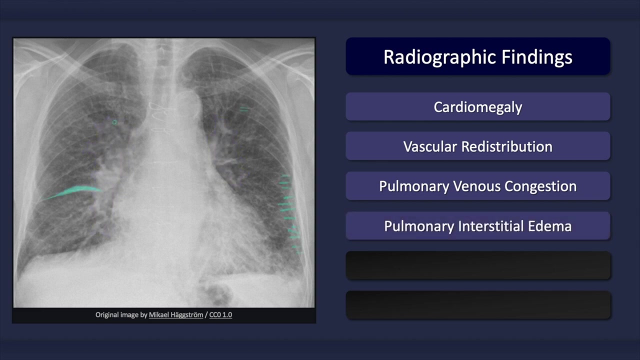 On an erect posterior-anterior chest. x-ray. suggestive findings include cardiomegaly, which does not necessarily need to be present. vascular redistribution, that is, the cephalization of blood flow. pulmonary venous congestion, pulmonary interstitial edema. 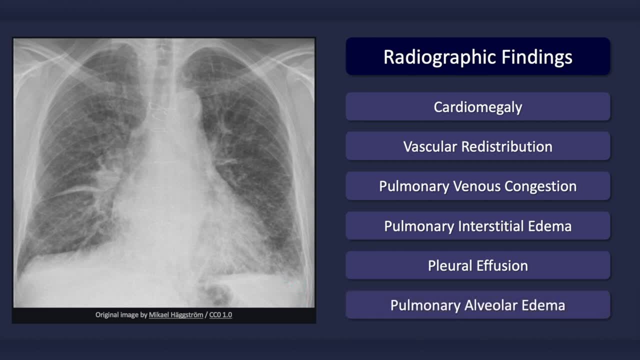 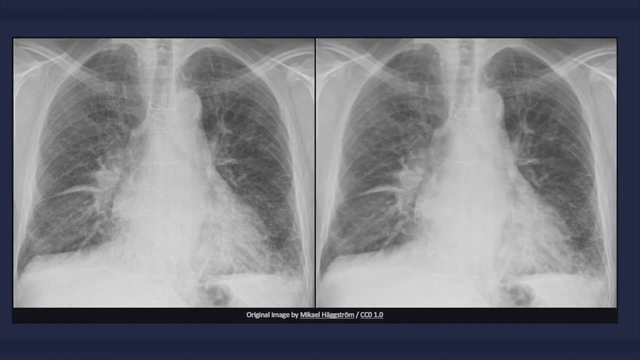 pleural effusions and, in more severe disease, alveolar edema, which is not clearly evident on this radiograph Cardiomegaly, particularly in concert with other findings, is a suggestive feature of congestive heart failure. However, keep in mind that congestive heart failure can occur in the presence of a normal cell. 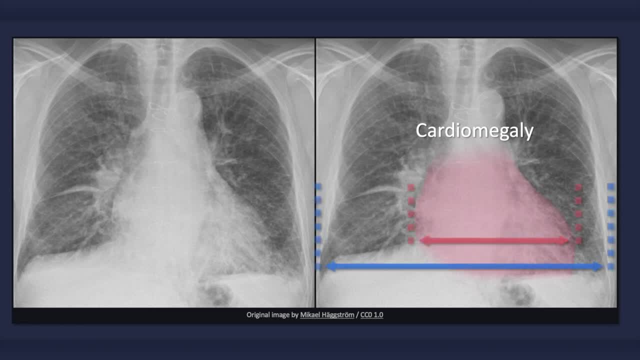 Cardiomegaly is said to be present when the cardiothoracic ratio is greater than 0.5.. That is when the largest transverse distance between the left and right heart borders of the cardiac silhouette is greater than half the width of the thorax. 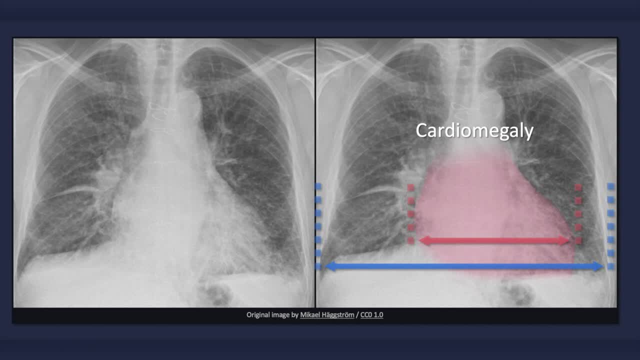 In this image, the cardiothoracic ratio is approximately 0.6.. Now you should also be aware that on anterior-posterior films, determination of heart size is unreliable due to magnification. Vascular redistribution is one of the first signs of congestive heart failure. 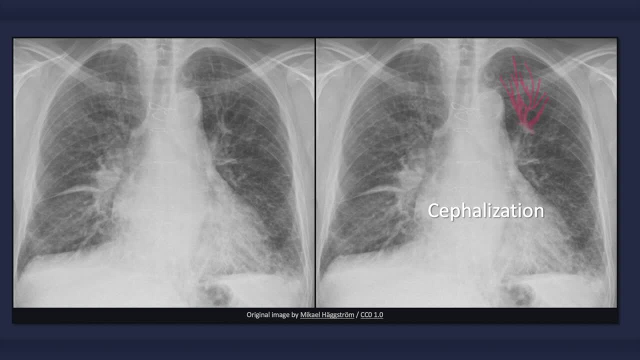 Increased blood flow to pulmonary vessels in the upper lung zones results in an increase in size relative to blood vessels in the lower lung zones. This caudal-to-cranial redistribution of blood flow should only be inspected for in an erect X-ray, since equalization of blood flow may occur in the supine position. 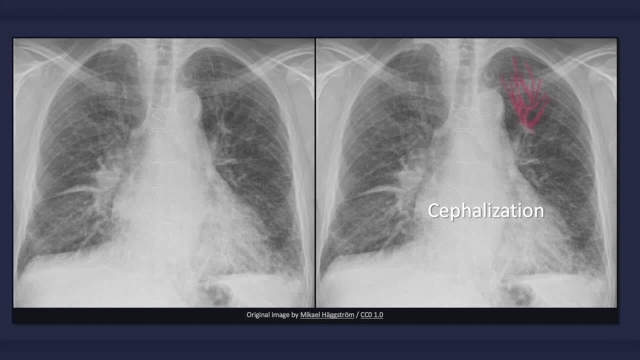 The finding of upper-low blood diversion, however, can be difficult to appreciate on a plain radiograph. One other way that blood flow may occur in the supine position. one other way that it can be identified is by the discovery of a superior-lobe artery. 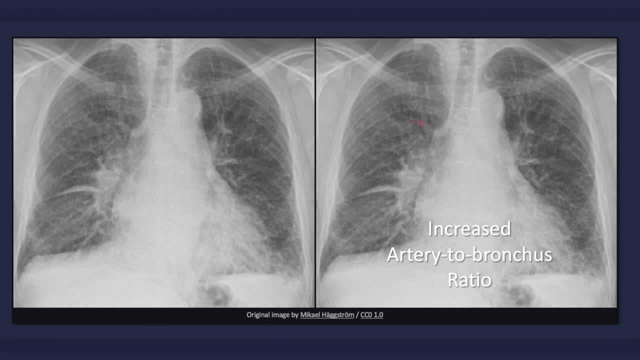 with a greater diameter than its accompanying bronchus. Now, since it is hard to be certain on this radiograph, this example should be taken for illustrative purposes. The bronchus is the ring-like structure with a hollow center, while the artery is filled in. 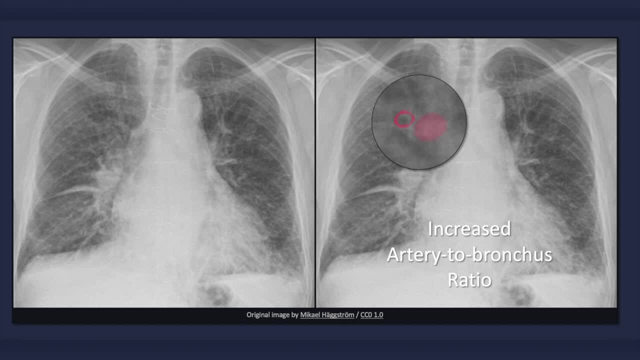 Normally the upper-lobe artery-to-bronchus ratio is less than 1 to 1.. Here the reverse is seen, with a larger artery than bronchus. You may have also noticed the prominence of the hilar region and the widening of the vascular pedicle in this radiograph. 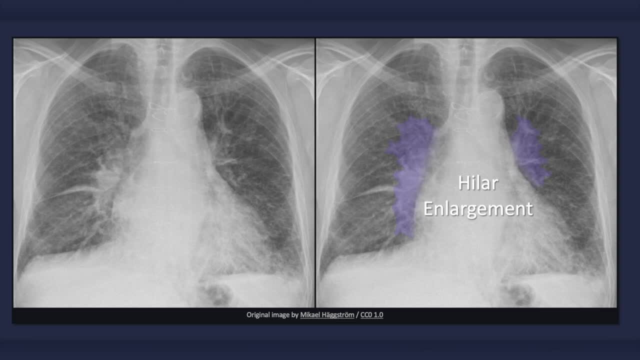 The fullness of the right hilum is particularly evident, whereas the left hilum is predominantly obscured by an enlarged cardiac silhouette, Unlike with lymph node enlargement, in which case the hilar can appear as a large lumpy mass. the hilar region in this X-ray has irregular borders. 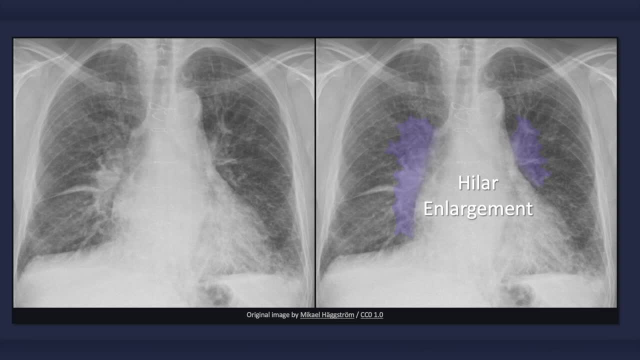 due to thickened outward branching vessels. The increase in hilar size, as well as the vascular pedicle widening in this X-ray, are due to pulmonary venous congestion. An edematous interstitium is another important feature of congestive heart failure. 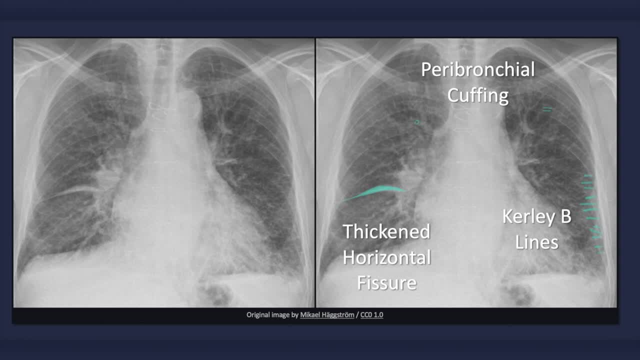 Three signs of thickened interstitial tissue include curly B-lines, peribronchial cuffing and interlobal fissure. thickening Curly B-lines are fine linear opacities that are only 1 to 2 mm in width. 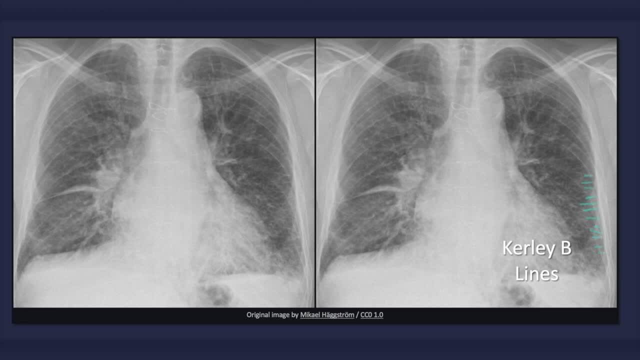 They are typically located peripherally in the lower lung fields near the costorphinic angles. When viewed close up, they can be seen to extend perpendicularly inwards from the pleura and are up to 3 cm in length. These opacities can also be seen head-on. 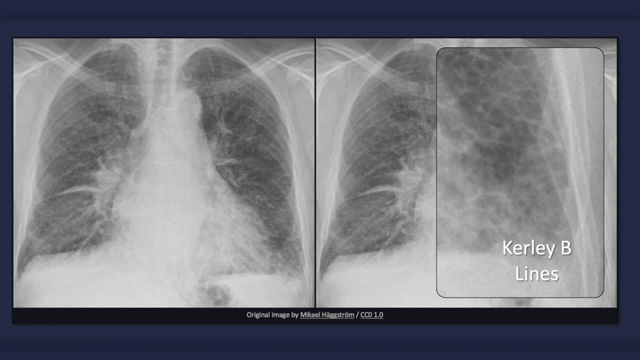 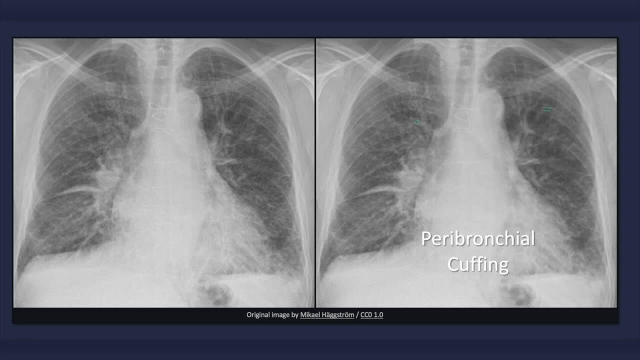 in which case they are referred to as curly C-lines, or radiating outward from the hilar, in which case they are called curly A-lines. Peribronchial cuffing is another discrete finding which occurs due to edema of the bronchial wall. 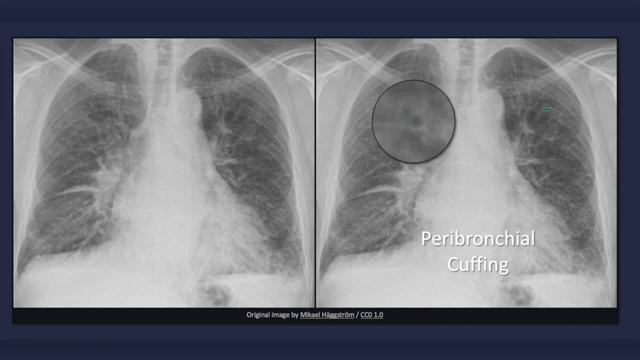 When viewed head-on, it appears as a donut or a ring. When viewed tangentially, that is, from the side, it appears as two parallel lines which to some extent resemble tram tracks. Note that peribronchial cuffing can occur in other conditions as well. 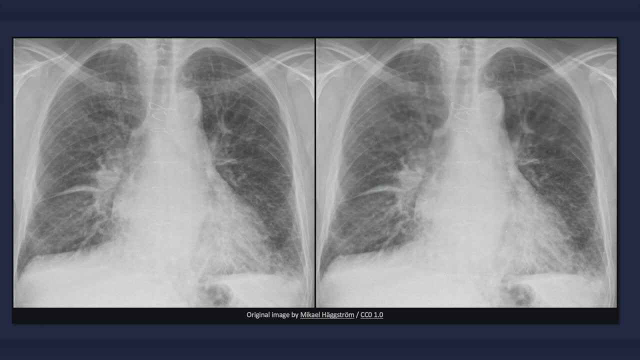 such as chronic bronchitis. Also evident in this image is a thickened minor, that is horizontal fissure. This finding is easier to detect on a lateral radiograph, where both the oblique and horizontal fissures may be visible Collectively. 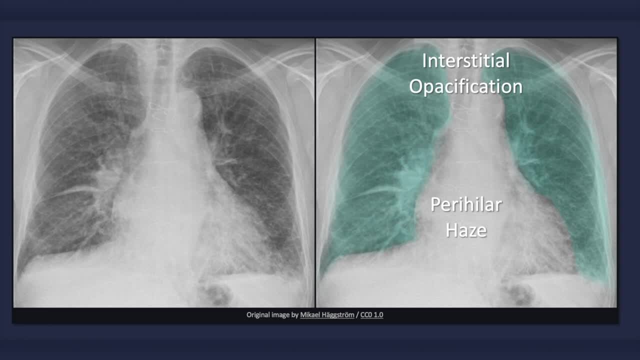 interstitial edema results in widespread blurring of lung markings. The loss of definition results in a hazy appearance of the lung fields and hilum bilaterally. Now let's turn our attention to the bottom right corner of the radiograph. Note that there is a decrease in definition of the left costorphinic angle. 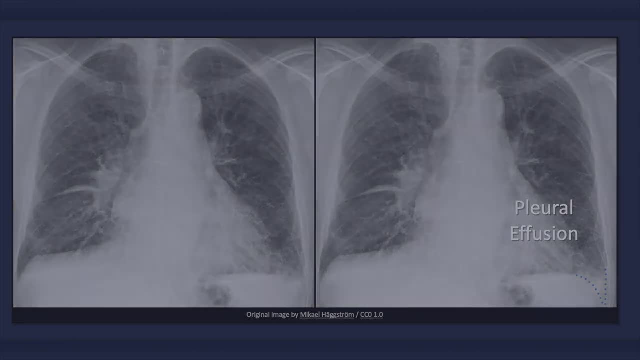 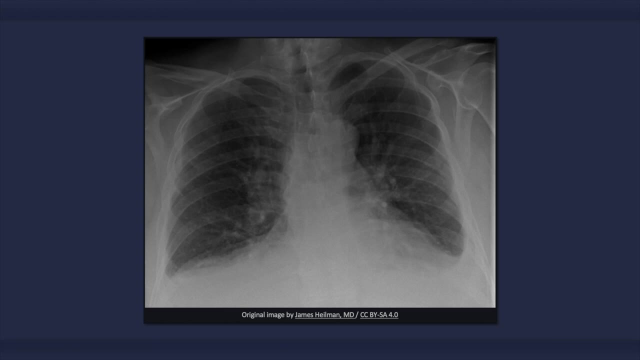 a finding that is consistent with a pleural effusion. Here is another X-ray of congestive heart failure. In this case, there are bilateral pleural effusions, which can be identified by the loss of costorphinic angles and obscured hemidiaphragms. 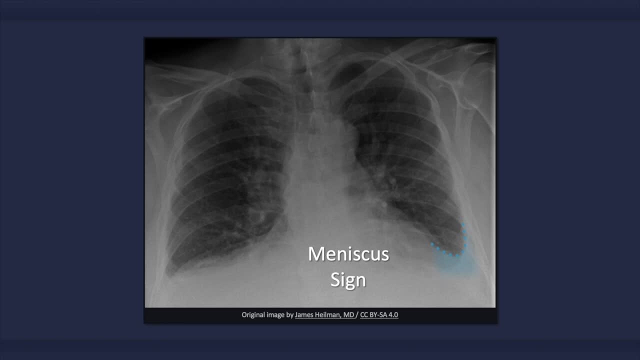 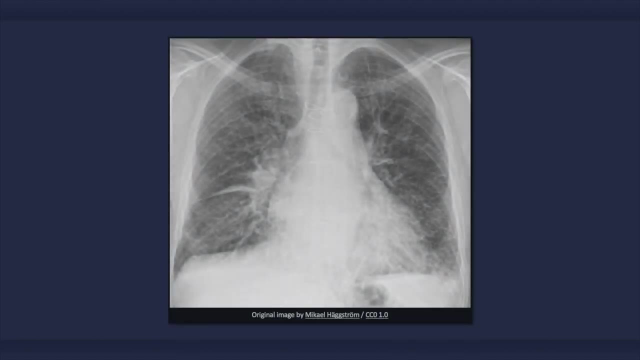 Below the left lung we see the meniscus sign, in which the opacity has a concave upper border and is higher laterally than medially. Alveolar edema is a more severe sign of congestive heart failure and is not clearly evident in this radiograph that we have thus far been examining. 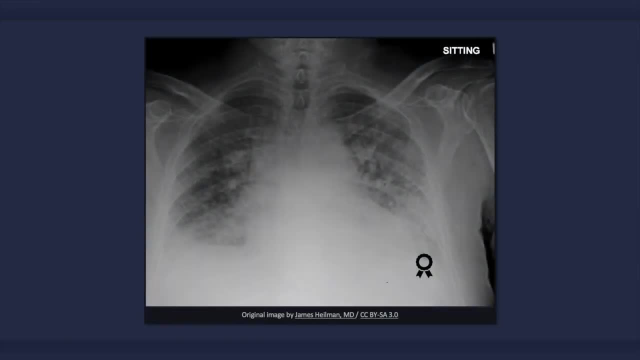 In this image, many of the aforementioned findings of congestive heart failure are present, plus alveolar edema which classically results in central and symmetrical air space. The outer third of the lung is frequently spared, resulting in a characteristic batwing configuration. 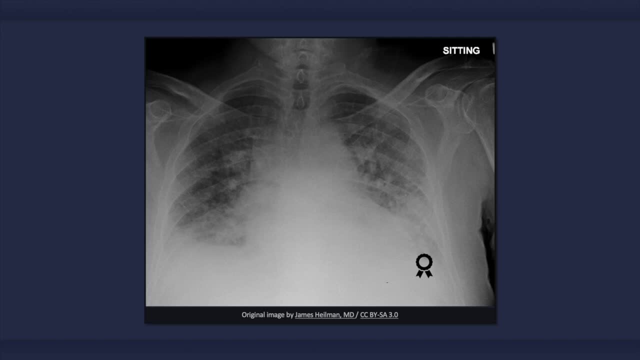 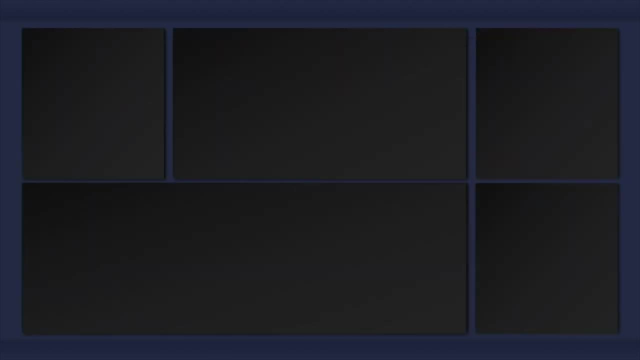 However, the patterns of pulmonary opacification are variable and can be more or less diffuse and asymmetric or patchy. To quickly recap, the plain radiographic findings that can occur with congestive heart failure include cardiomegaly. signs of vascular redistribution, such as cephalization. 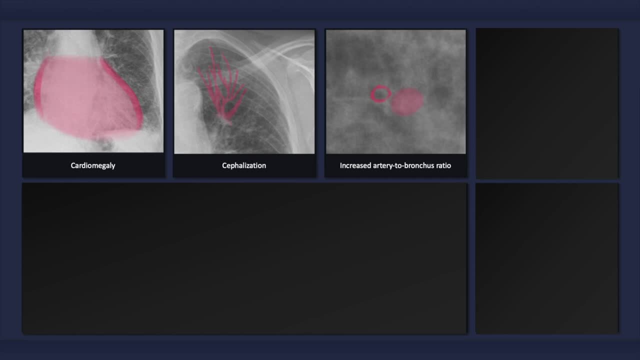 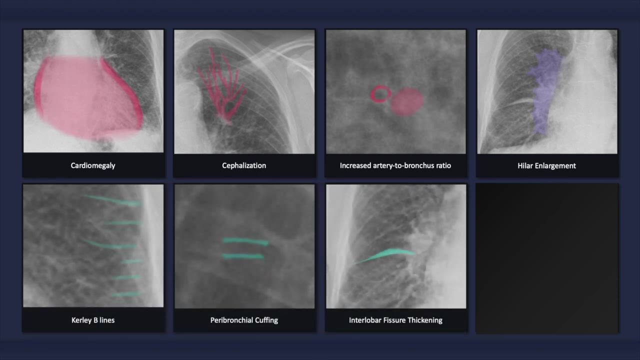 and increased artery-to-bronchus ratio and superior segments. signs of pulmonary vascular congestion, such as hilar enlargement and a widened vascular pedicle. signs of pulmonary interstitial edema, such as curly B-lines, peribronchial cuffing and interlobal fissure thickening. 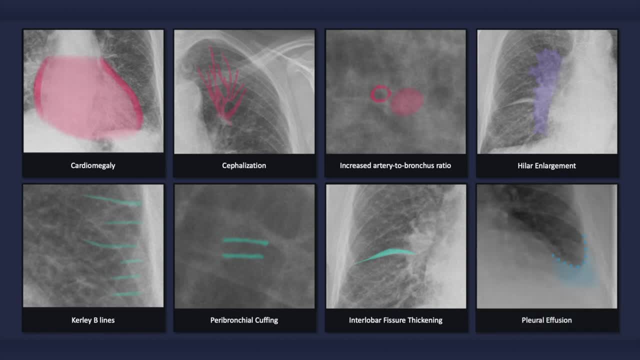 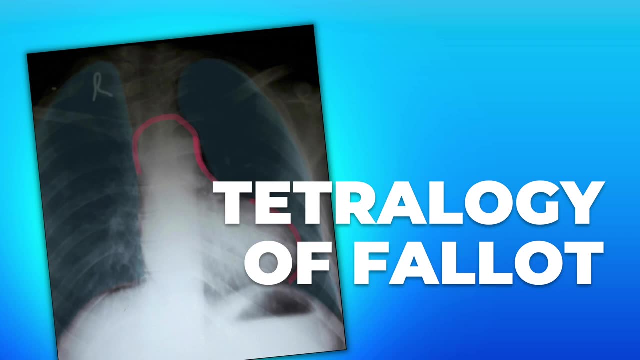 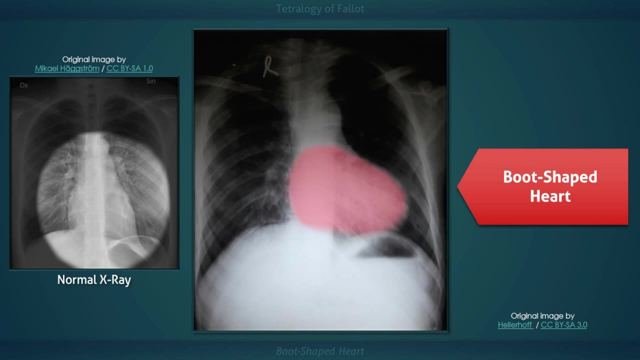 pleural effusions and, in more severe cases, alveolar edema. The term boot-shaped heart refers to the abnormal appearance of the cardiac silhouette. Two of the four classic defects that contribute to this appearance are a ventricular septal defect and pulmonic stenosis. 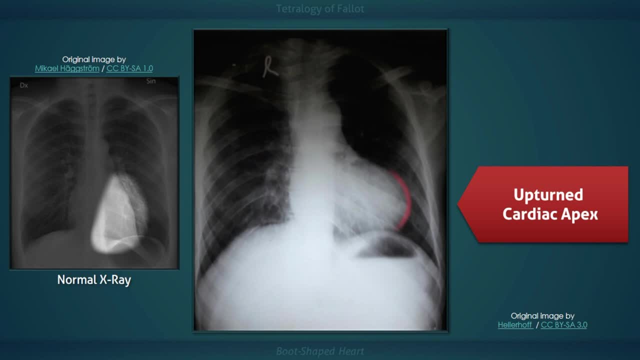 This combination of defects results in an elevated right ventricular systolic pressure, with ensuing right ventricular hypertrophy, which is a third defect in the classic tetralogy. In this radiograph, right ventricular hypertrophy has resulted in an upturned cardiac apex. 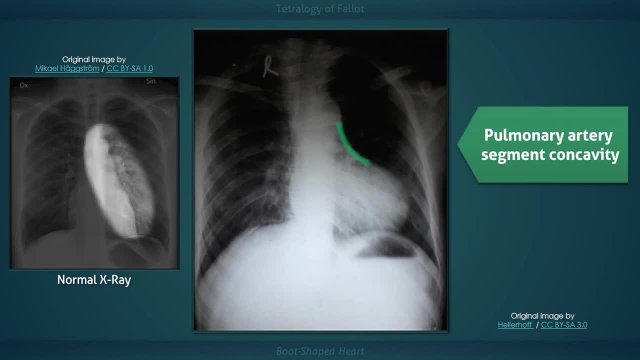 that is positioned abnormally high above the diaphragm. Pulmonic stenosis can also result in a small main pulmonary artery due to decreased flow. This finding is depicted on the x-ray as an increased concavity of the main pulmonary artery segment. 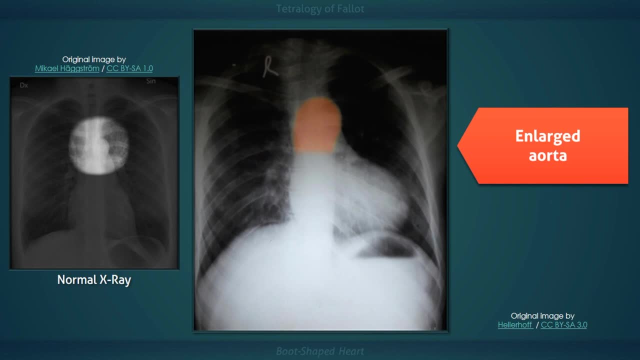 The fourth defect is an overriding aorta which, along with pulmonic stenosis and a VSD, facilitates the shunting of blood away from the pulmonary system. This results in a large aorta which, in a significant proportion of patients, is right-sided. 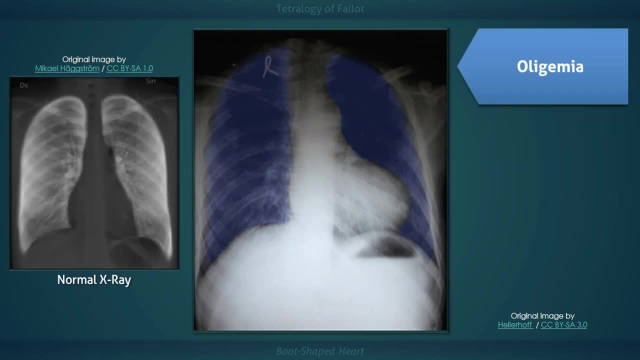 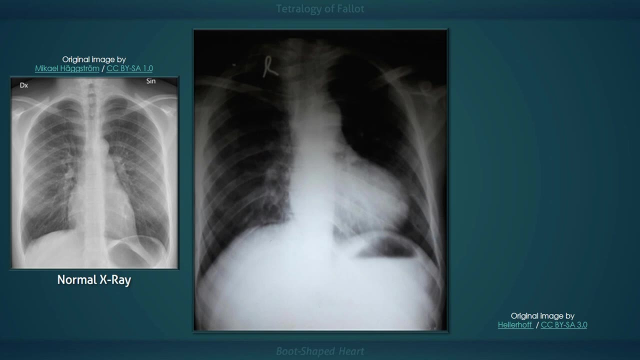 and decreased pulmonary vascularity, which is visualized on the x-ray. On this x-ray is diminished lung markings, that is, increased blackness of the lung fields. Now for a quick review. The four findings in this radiograph of a boot-shaped heart include: 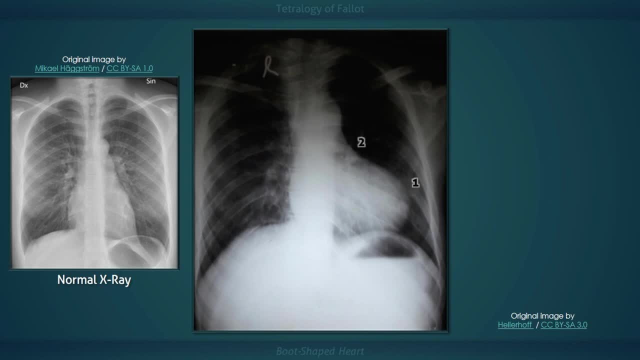 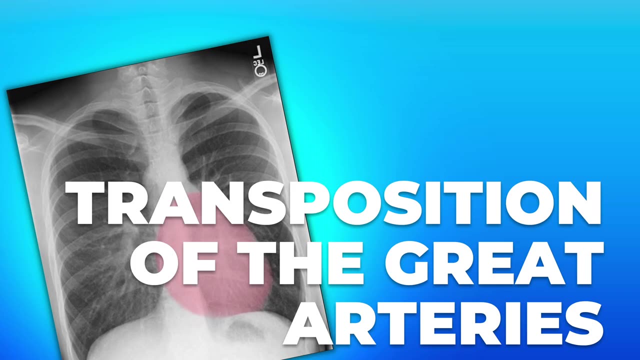 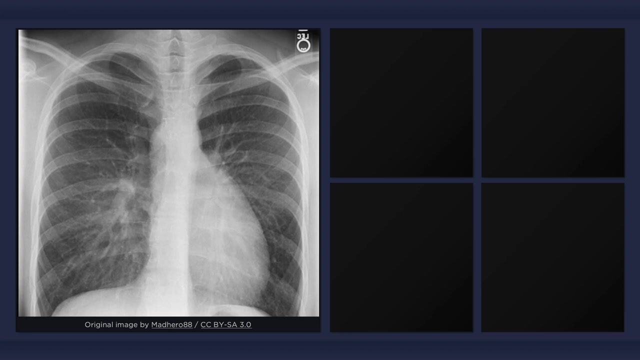 an upturned cardiac apex, a concaved main pulmonary artery segment, an enlarged aorta and a leukemia. In this example, the first abnormality that may come to your attention is the globular, or oval-shaped cardiac silhouette. The unusual heart shadow occurs due to prominence of the right atrium. 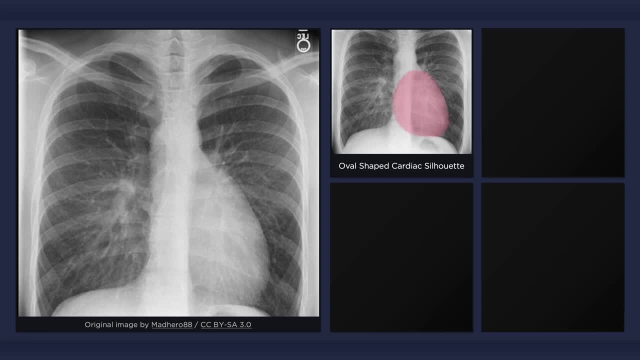 and convexity of the left ventricle. In more classic examples, the right atrium protrudes out more laterally and the oval shape of the heart looks like it's tilted sideways. The second abnormal finding is a narrow vascular pedicle. 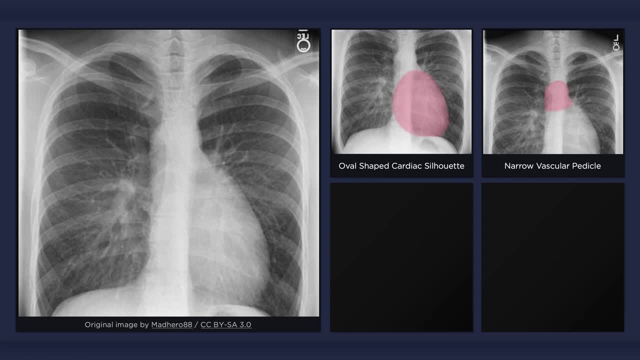 This occurs because the thymic shadow is typically small or absent and the pulmonary artery lies directly behind the aorta. On a lateral radiograph, however, this front-to-back orientation of the aorta and pulmonary artery would result in a wide superior mediastinum. 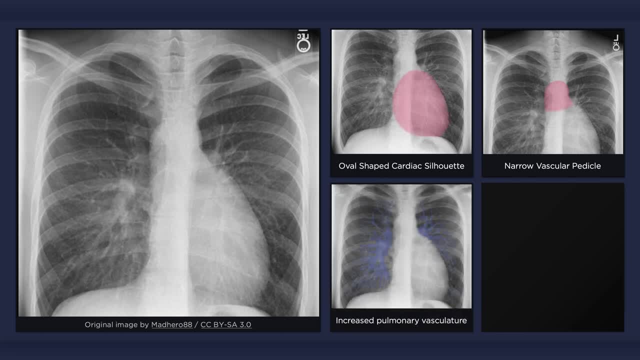 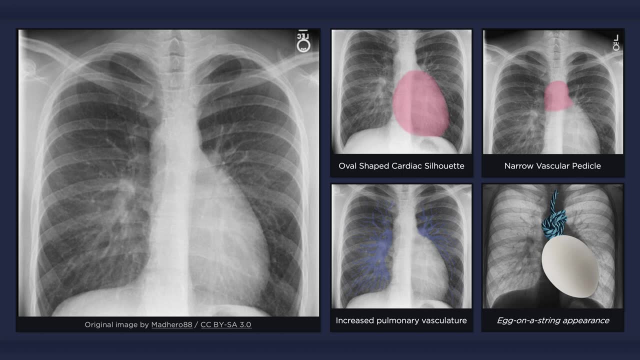 Overcirculation of pulmonary blood flow results in a third finding, represented on plane radiography as an increase in vascular lung markings. The combination of an oval cardiac silhouette and a narrow vascular pedicle has been visually described as an egg on a string. Now, while the combination of these findings 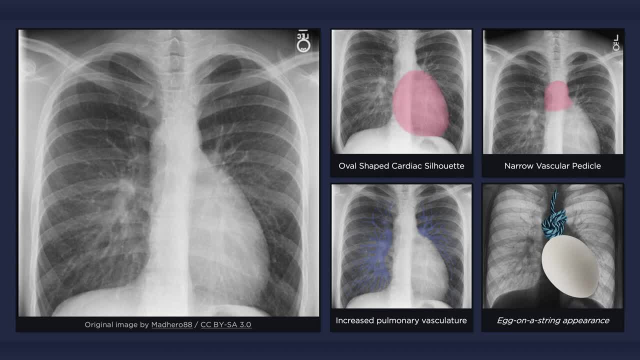 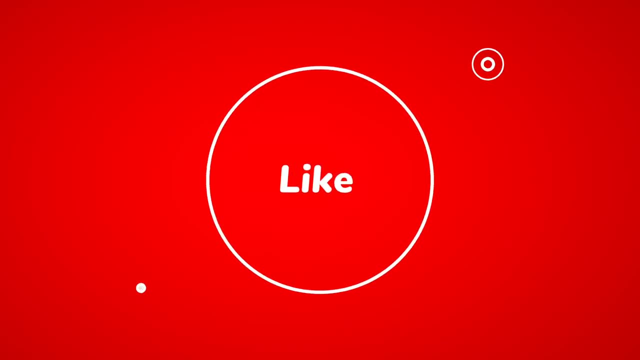 results in a classic appearance. it is important to keep in mind that in many cases, the x-ray is completely normal. Thank you for watching.